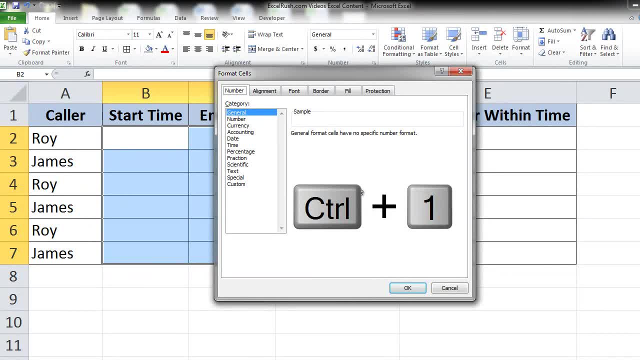 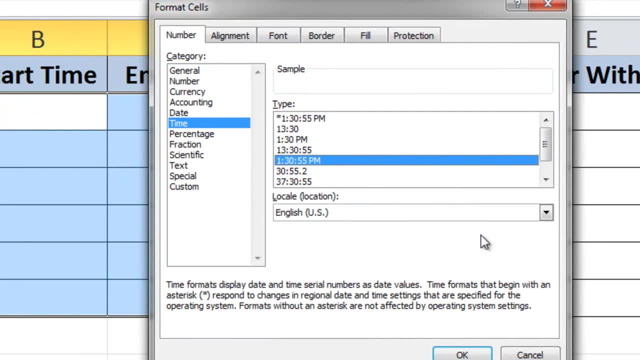 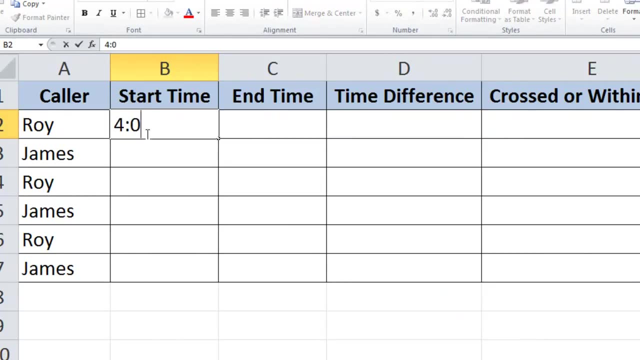 go to this particular box of format cells using the shortcut control plus one Here. go to time and I like this format. you can choose it too and press ok. Let's enter a sample time: 4 pm. As soon as I press tab automatically, it's taken the format that I wanted Here. I. 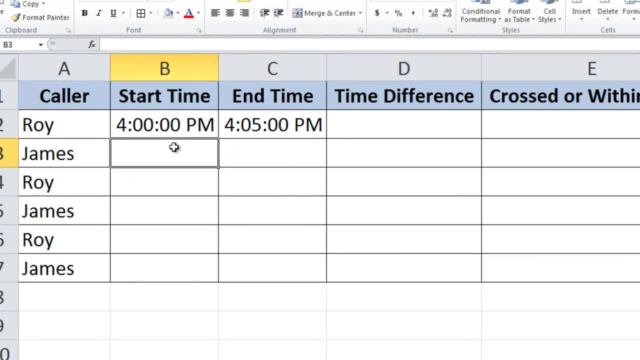 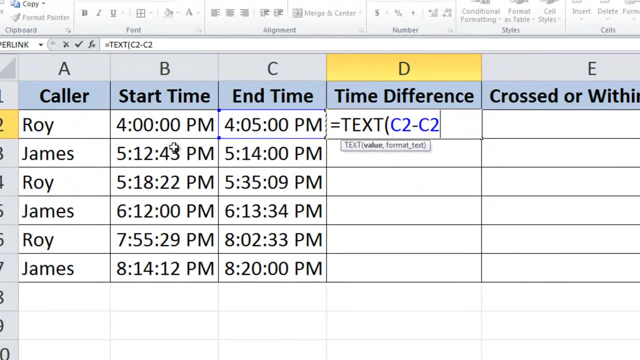 am saying end time is 4.05 pm. Similarly, fill more data. Now let's calculate the time difference between the two times using equal to text. formula Equal to text. Take the end time first, minus the start time comma. put the format text as: 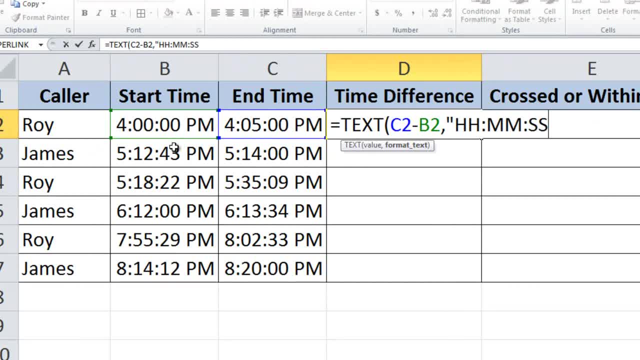 hh. colon mm. colon ss. in double quotes, close the bracket. This is for hours, minutes and seconds. Press enter Wow, So in one shot we know that the exact time difference between these two times is 5 minutes and 0 seconds. Let's copy this formula down. We got for each. 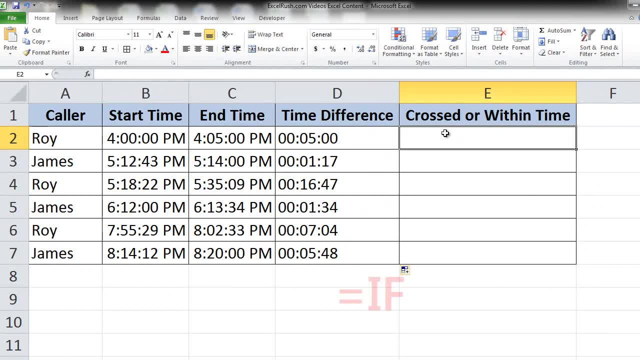 of them. Now let's add some insights to our data. using the formula equal to if. What we want to know is whether the customer service executive has resolved a particular issue on the phone in 5 minutes, or has he crossed 5 minutes? So basically, 5 minutes is something which 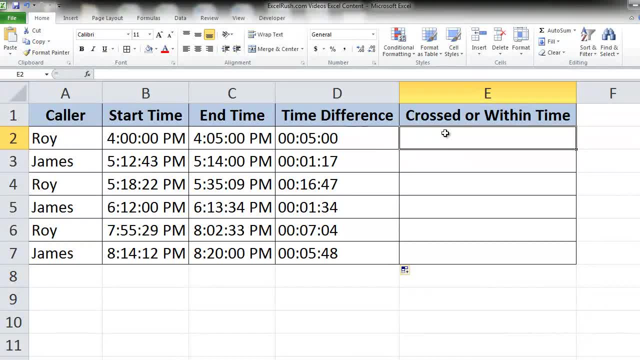 is acceptable. Beyond, that is not very good for his ratings. How do we measure this? Thus, to see if he has crossed the time difference. So, in order to measure the time difference between the two times, we need to basically check three parameters. If the number of hours is more than 0, he has crossed it. If 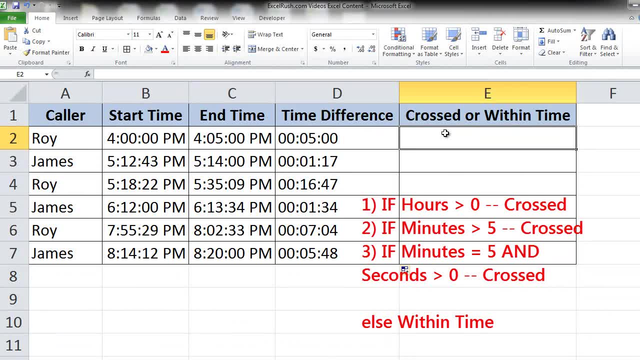 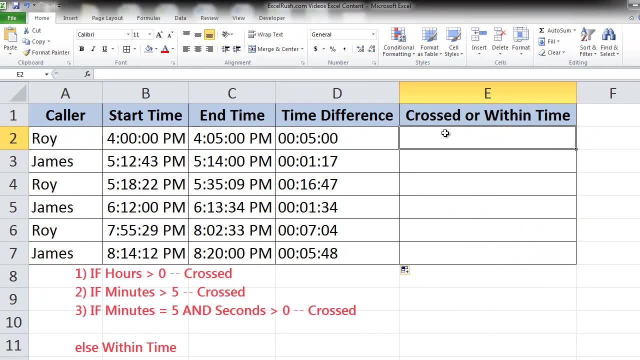 the number of minutes is more than 5, again, he has crossed it. If the number of minutes is 5 but the number of seconds is more than 0, he has again crossed it, Or else he is within the time. Yes, easy to understand. Let's put the formula Equal to if Let's 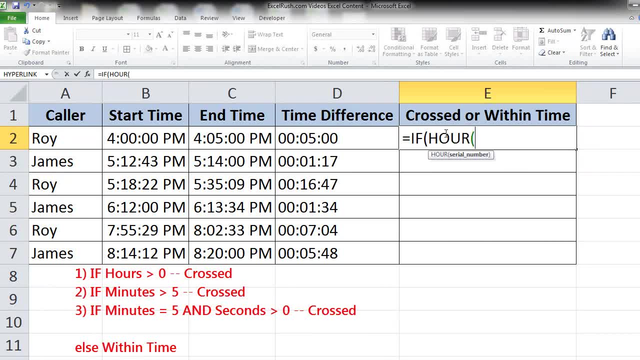 take the first condition: If the number of hours is more than 0, he has crossed it. If the number of minutes is more than 0, he has crossed it. So we want to check whether the hour of this particular time is more than 0. That's our first condition. If it is, we. 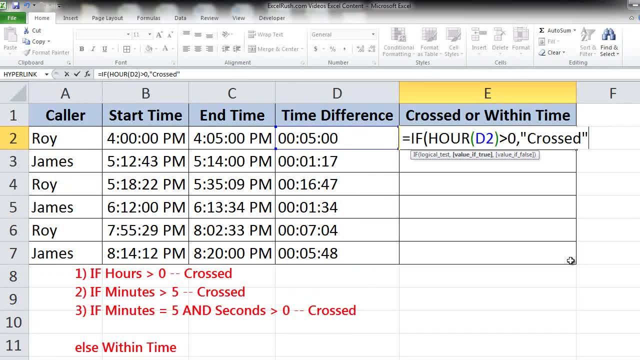 want to say crossed comma. Now, the first condition has been checked. Now the second condition will have to be put in the value, if false, of the if formula, which we can also call as nested if, If, under if. So, for the second condition, we have to put in the value: 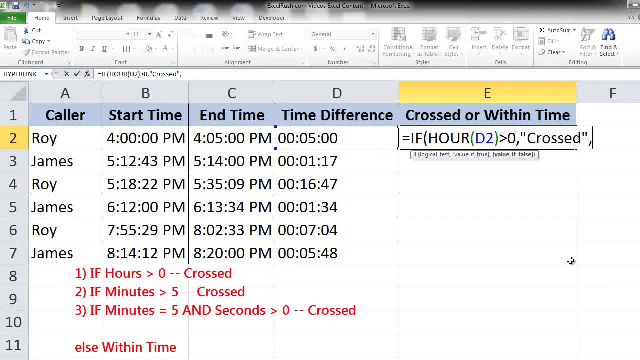 if false of the if formula, which we can also call as nested if, If under. if So, for the second condition, we put if again and we check minute of this particular cell to be more than 5.. Are you getting it? It's very simple. Basically, the formula if has three. 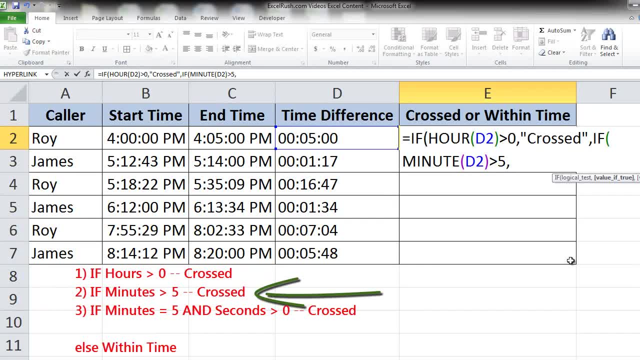 things: First the condition, then the value of true, then the value of false. So once we mention the condition, a condition can either be true or either be false. right, If the condition is true, we want the word crossed. So if he has crossed it, we can either. 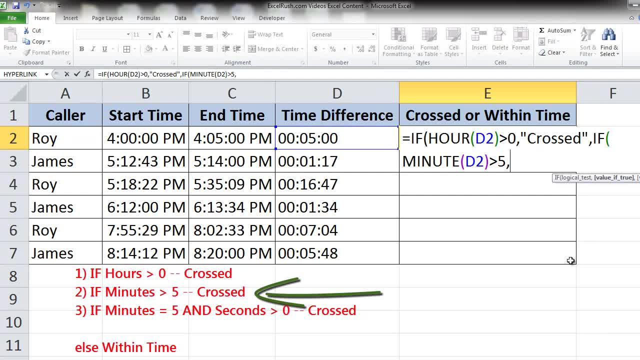 word crossed to appear. If it is false, we want to check the next condition. as simple as that. So the second condition is what we mentioned: minutes more than five comma. again, we write crossed. For the third condition, we have to check two things: whether the minutes, 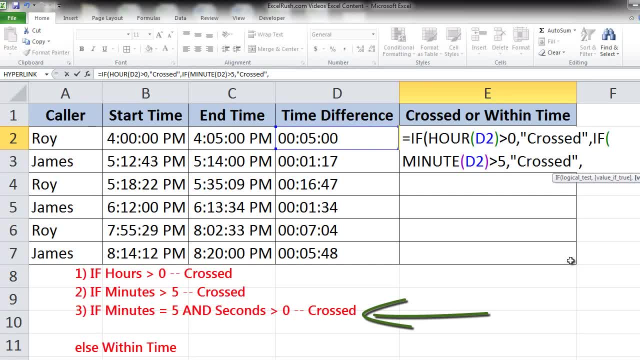 is equal to five and the number of seconds is more than zero. So here we will have to say if and minutes of this particular cell is equal to five, comma second of this particular cell is more than zero. Close the bracket for the and comma crossed again, or else now. 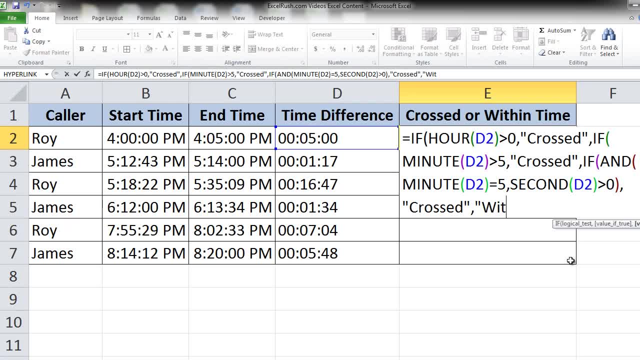 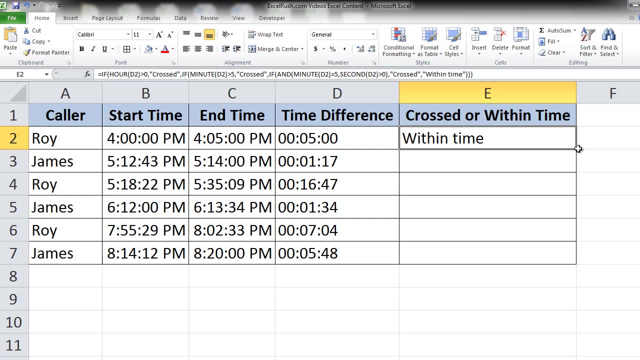 all our conditions are over. So then we can say in double quotes: within time, that is our value of false And close, the number of brackets required for the if and press enter. So Roy, in his first call, has completed in exactly five minutes. That's why it says within time, Let's copy. 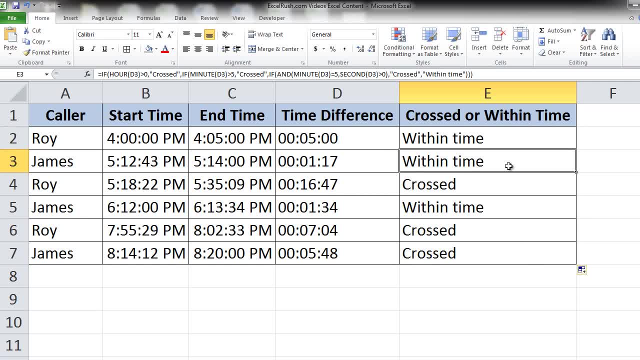 this formula down and check Superb For James's first call, it's within time one minute and seventeen seconds. Roy, sixteen minutes and forty seven seconds, So he's crossed the time limit, and so forth. Let's also add some insights using conditional.